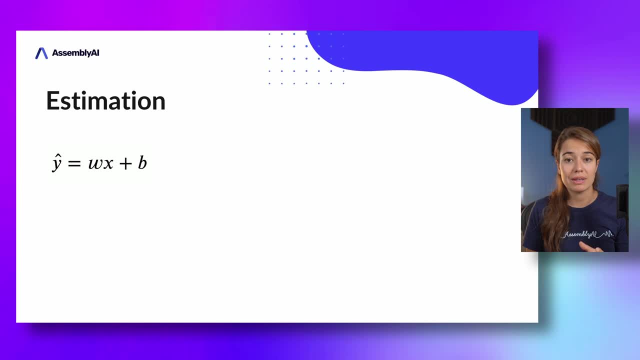 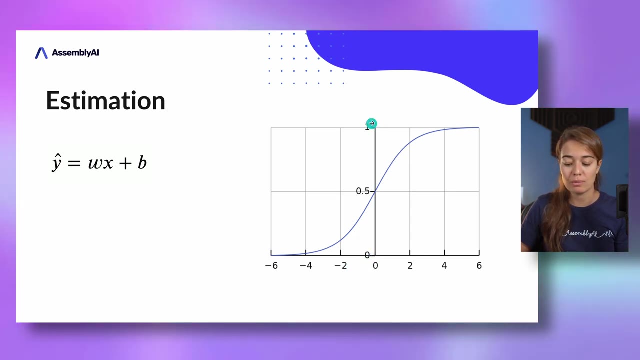 logistic regression. what we're trying to do is to create probabilities instead of a specific value, and to do that, what we're going to do is to put in our value inside the sigmoid function that looks like this, and then get a probability distribution that will be between 0 and 1, and 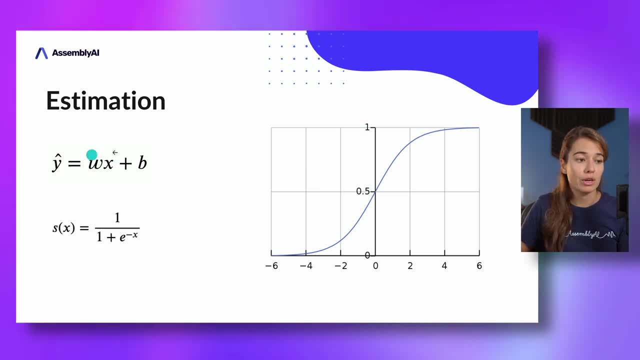 this is how the sigmoid function is calculated, so our equation goes from this to this. and to make it easier, we also call this equation with an h, so in the coming pages you might see it depicted as this. so don't just don't get confused With logistic regression instead of using the mean squared error. 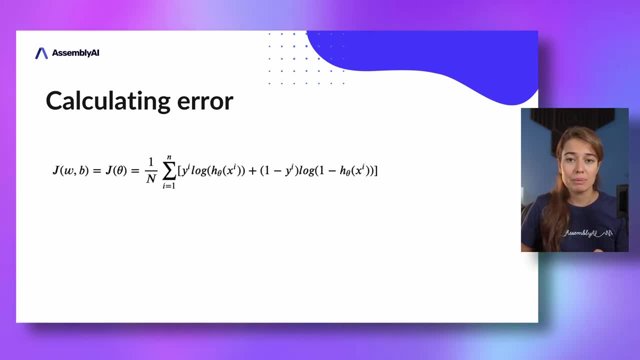 we're using something called cross entropy, so it's a little bit more complicated than what we have time for this video. so if you want to learn about how cross entropy works other than this equation that you see in front of you, you can go ahead and check that now. 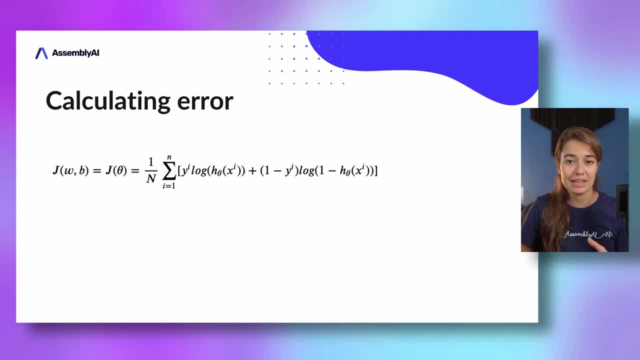 Again, we do the same thing. for logistic regression, we need to use gradient descent. and to use gradient descent, we need to calculate the gradient of this error function in terms of the weight and the bias. and this is how it looks like. again, very simple. we just jump to the end. 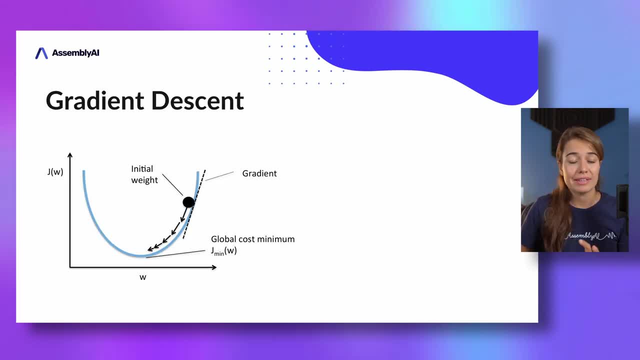 so that we can implement this in our code Very quickly again. what gradient descent is, we see, is a graph that shows us, given a parameter value, a weight value, what the error is. and this is their relationship. gradient descent tells us, given at any point of where we are in. 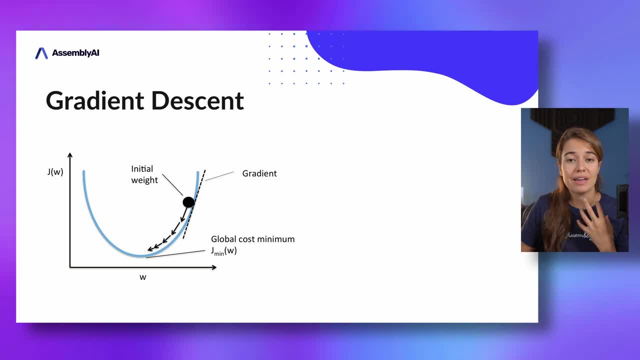 this graph which direction to go to minimize the error. once we know the direction that we need to go to through the gradients, what we do is we update the parameters, so the weight and the bias, by subtracting from the current value of the weight the gradient multiplied by the. 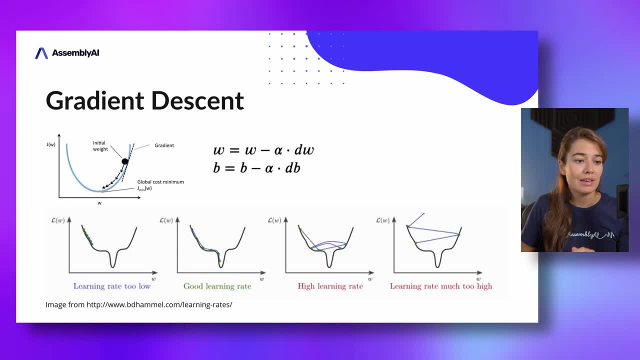 learning rate and again to quickly recap what the learning rate is is tells us how fast to approach in this direction or how fast to go in this direction. that gradient tells us, gradient descent tells us to go. so if you go too slow then you will make progress very slowly and you will 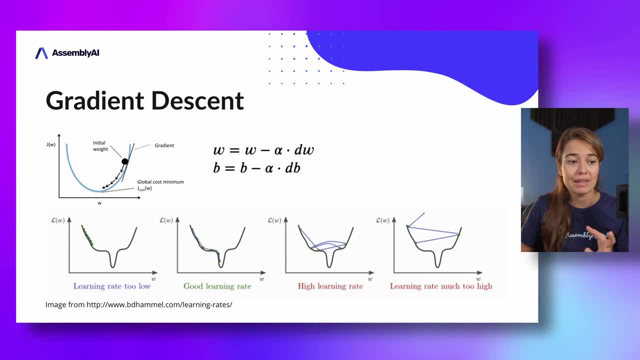 not be able to, or you might not be able to, make it to your minima in time. it might take too long, but if your learning rate is too high then you might keep missing your minima by jumping around. but if you choose a good learning rate you might be able to make it to your minimum in time. 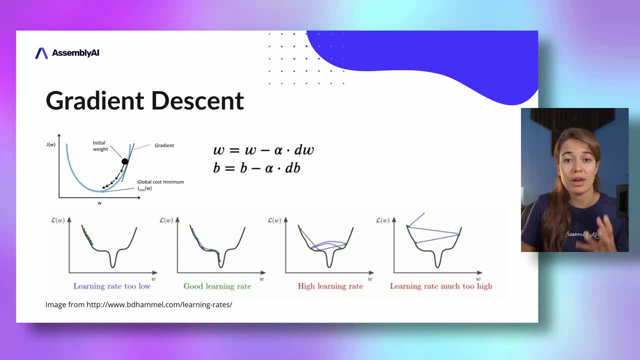 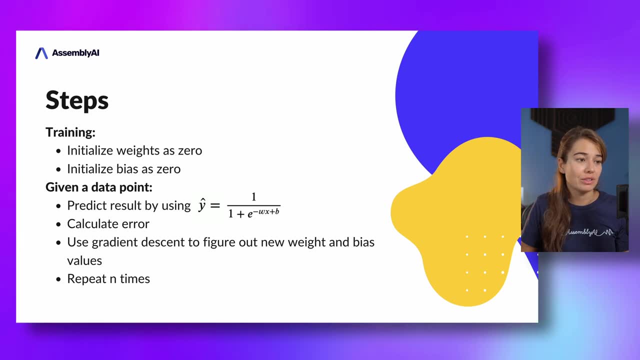 so if you choose a good learning rate, very likely you will eventually reach a point where your error is minimum. so to recap, in logistic regression, very similar to linear regression, what we do is at first we initialize the weights and the bias and then we predict or estimate a result using this equation. then we calculate the error and 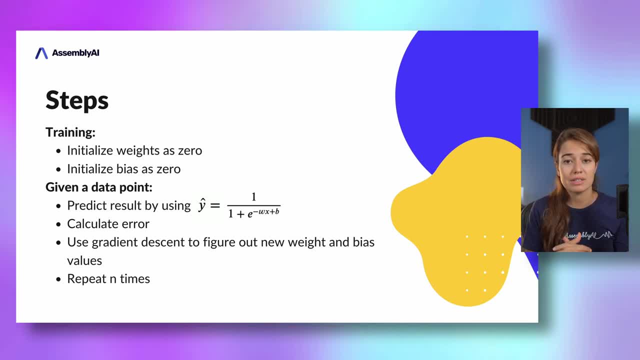 on top of this error, or using this error, we use gradient descent to figure out in which direction to change our weights and biases, also including our learning rate, and then we repeat this error, this process, number of times that the model creator told us to do so And during testing. 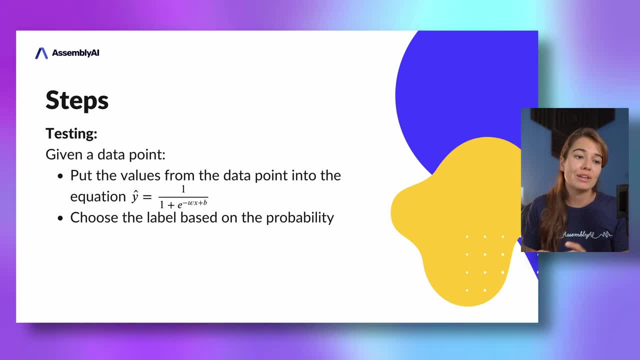 given a data point. we put the values that we get from the data point inside this equation and then, after we calculate this probability value, we choose a label that is based on the highest probability. So let's start implementing it now. All right, so let's start with the. 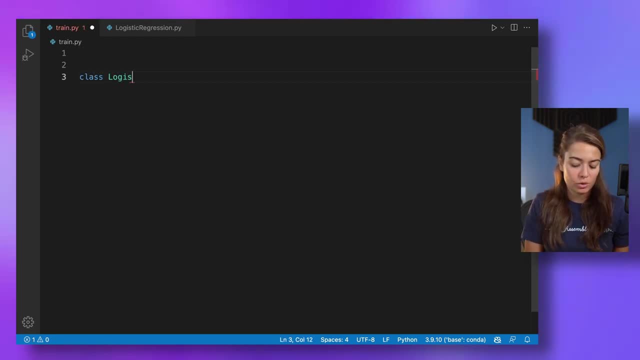 implementation. It's actually going to be quite similar to linear regression, but let's do it from the beginning. It's not going to take that long anyways. So at first, of course, I need an initialization function here. We need to pass the learning rate again and a number of iterations. 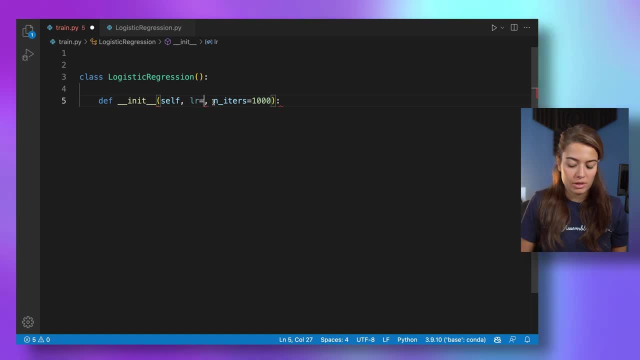 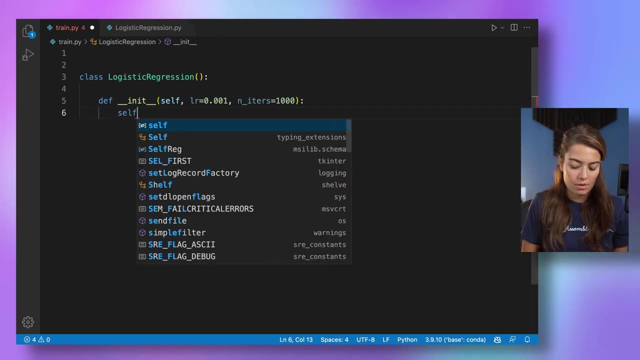 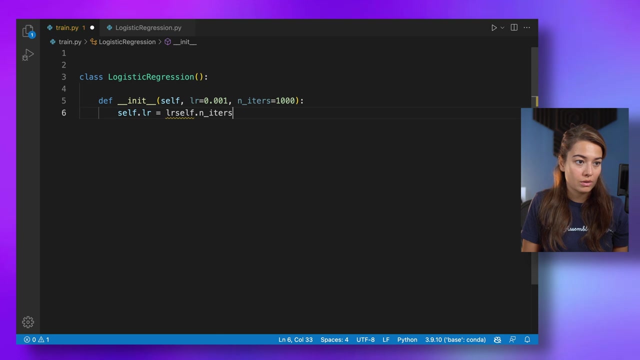 Number of iterations. we can again say like 100,000.. The learning rate could again be 0.001.. And we need a learning rate. it'll be learning rate. we need the number of iterations. Oops, Number of iterations is going to be number of iterations. And again we need the weights. 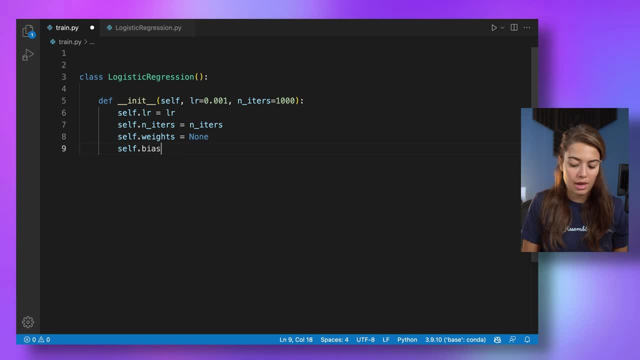 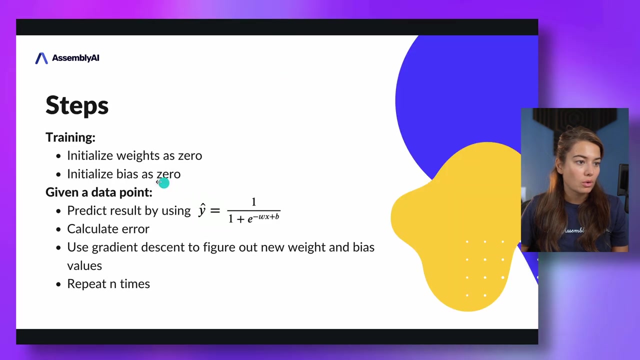 For now it'll be none And we need the bias. again will be none, And then I need another fit function And a predict function. So I will pass the x and the y to the fit function. Let's remember what we did for logistic regression. So initialize the weights and bias as zero, So we can do that again. 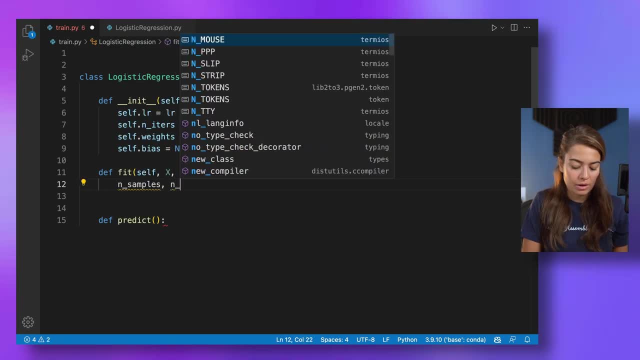 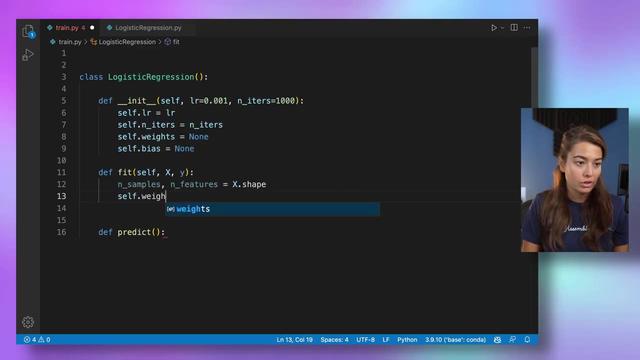 If you remember, we first need to get the number of samples and the number of features, And that's that we're going to get from x shape, And then I'm going to create the or initialize the weights, or at least assign zeros as weights, as going to be features need to. 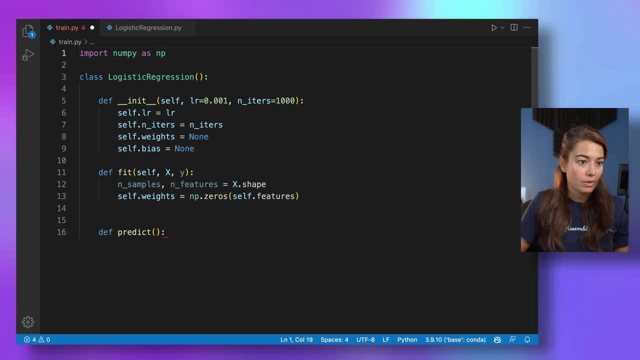 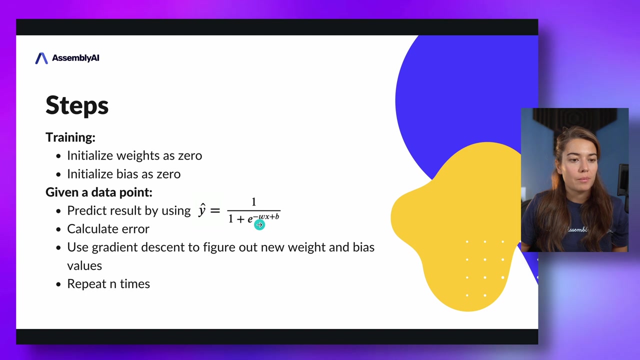 import non pi, of course, and the bias just as zero. Next thing that we need to do: predict the results using this calculation. Well, this is basically what we did with Linux. This is basically what we did with Linux: regression. so weights times the X values plus the bias put into a sigmoid. 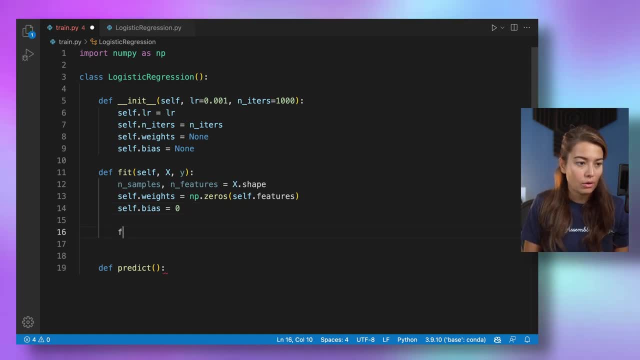 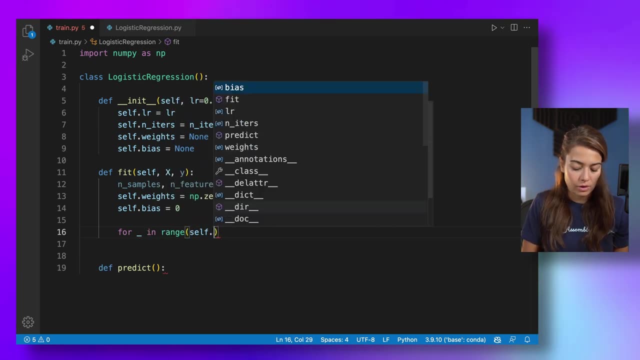 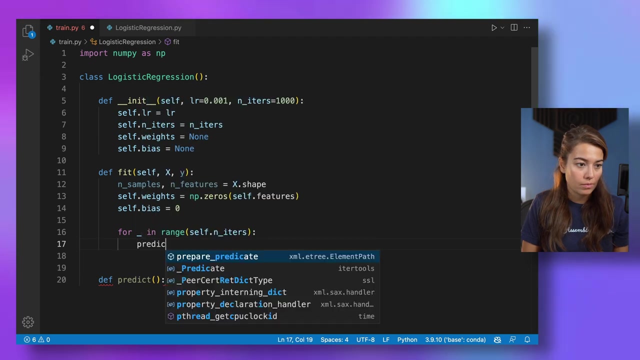 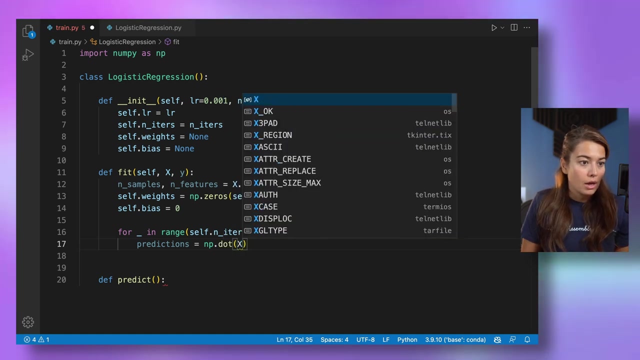 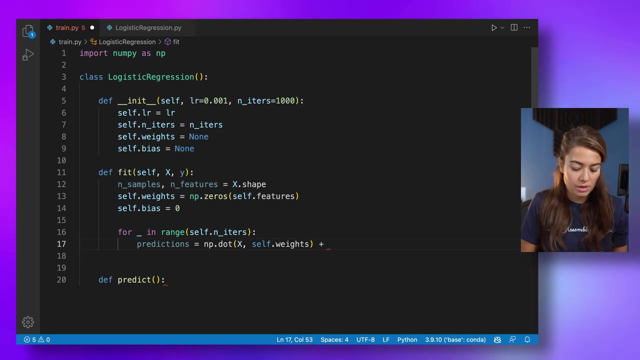 function. So that can be what we're doing. I already write the iterations, so we need to do it for number of iterations or a number of iterations times, this whole part here, and I will calculate the predictions: numpy dot of X that we pass here and self weights plus the bias. Maybe I can. 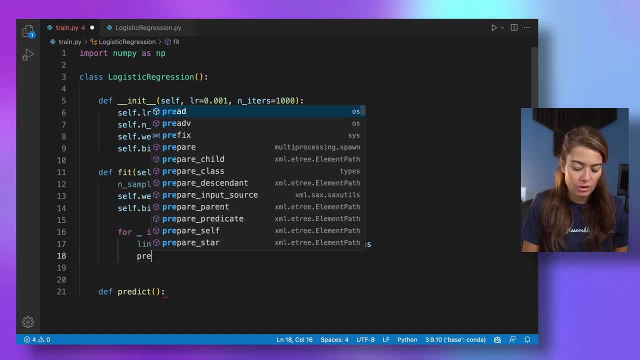 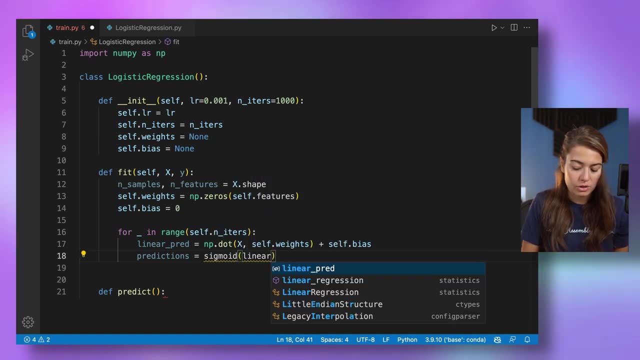 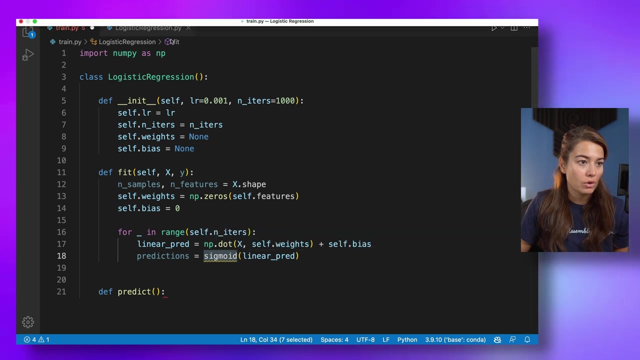 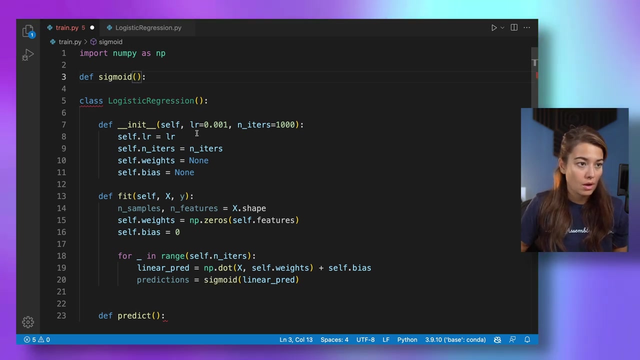 call this linear predictions, and then the actual predictions will be a sigmoid function and linear predictions inside it. So I need to create the sigmoid function. So let's do that. Maybe let's say sigmoid. What I need to pass it are some values. So let's refresh our memory What the sigmoid 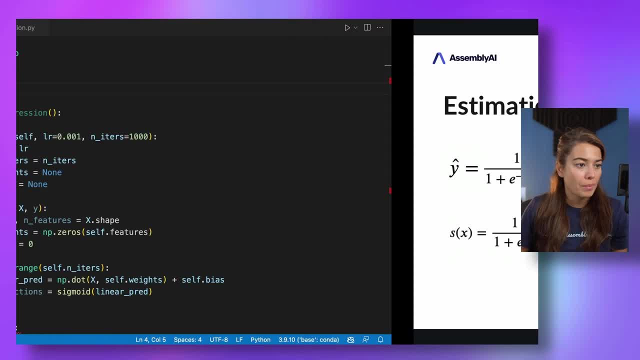 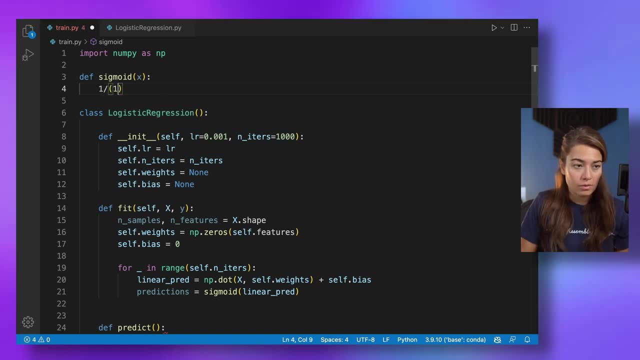 function look like 1 over 1 plus e over minus X. So this is what we can do: 1 over 1 plus exponential minus X, and that's all we need to do actually to calculate the sigmoid. So we'll do it here and then we call it here, and now we have the predictions. 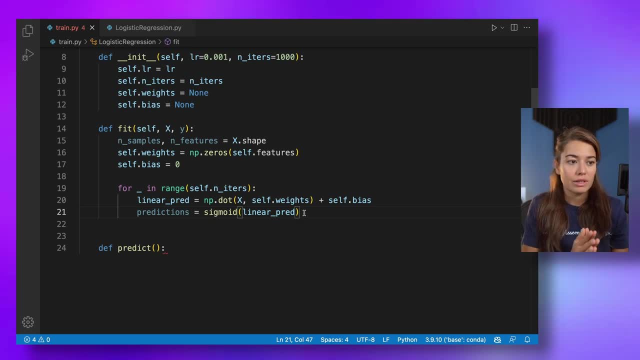 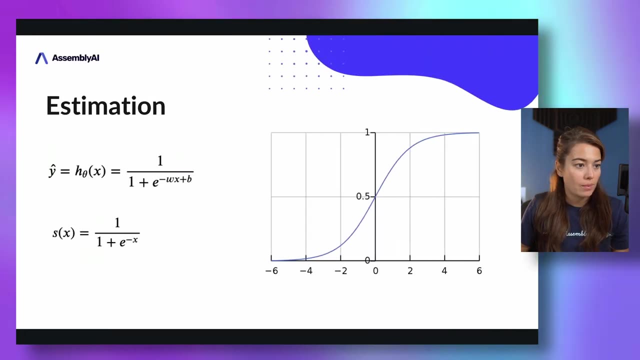 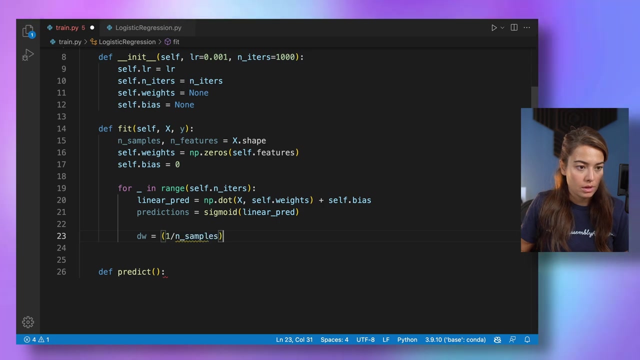 After we have the predictions, the next thing that we want to do is to calculate the gradients, and that's exactly the same as last time. So let's refresh our memory, All right. 1 over the number of samples. 1 over the number of samples. 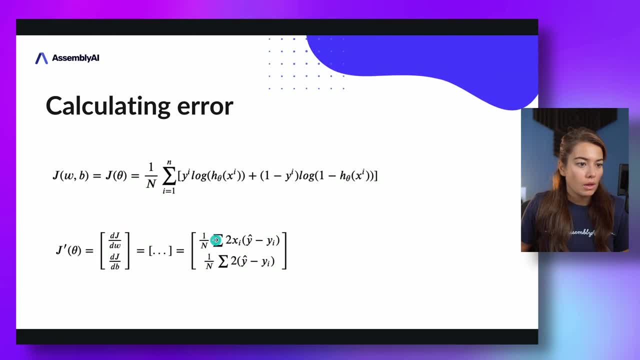 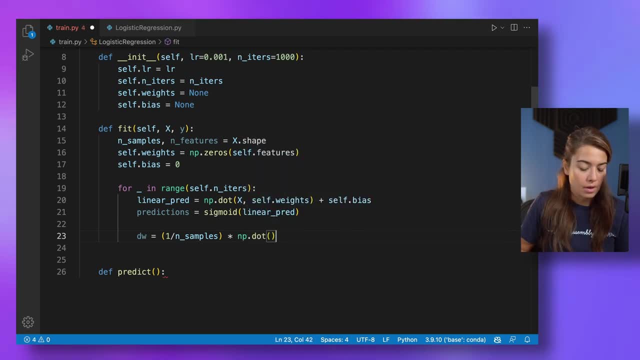 times the dot product We're going to get of X. but we need to get a transpose of X to be able to do the dot product, because otherwise the dimensions don't work, and the difference between the predictions and the actual Y. So that's DW. and to calculate the gradient for the bias you do 1 over a number of sample. 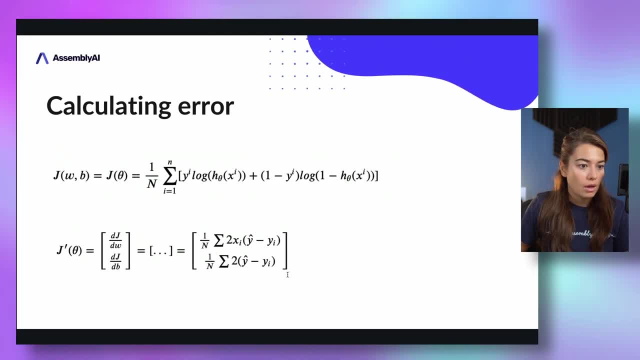 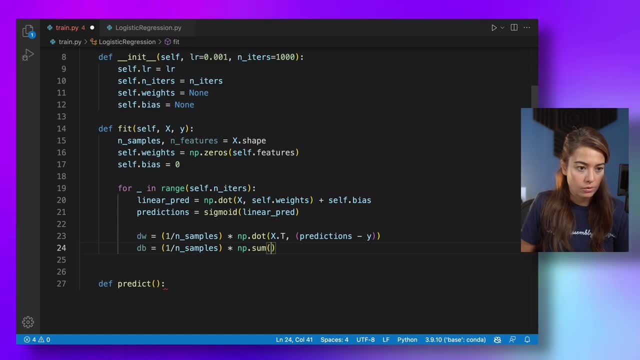 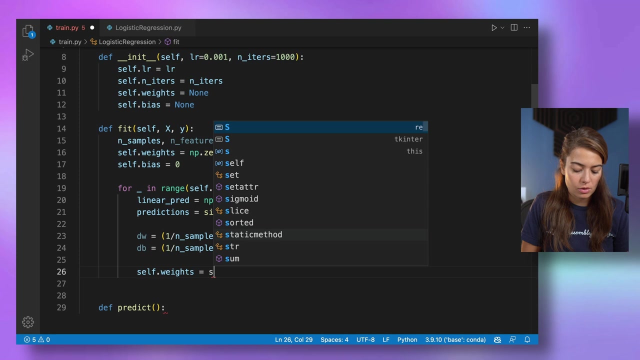 again times. let's see for that. we're not going to use a dot product. we're going to use the summation of predictions- predictions minus y and that's it- and to do the updates. I think we're going to do the same thing. yeah, exactly so. self weights equals to self weights minus. 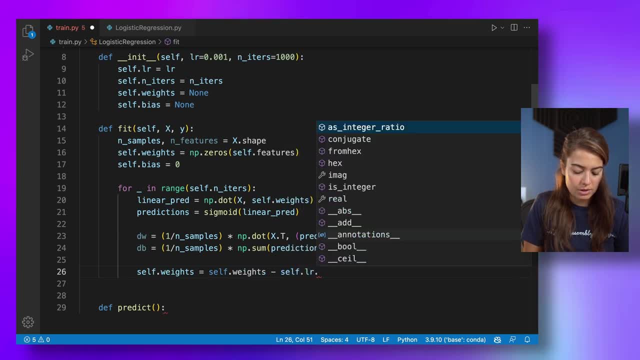 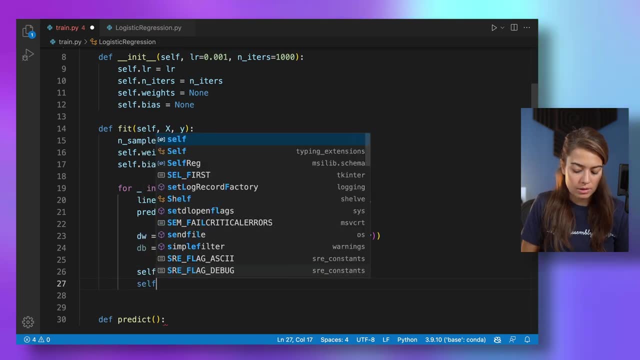 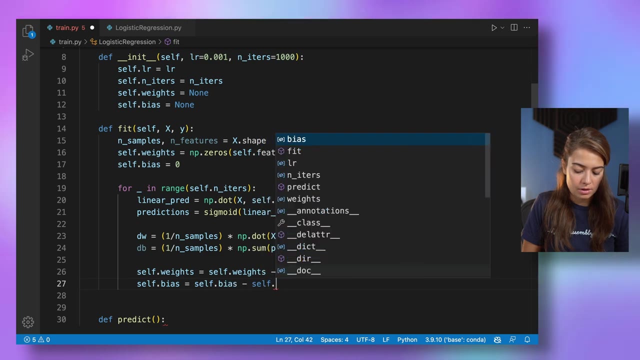 learning rate times d, dw and self bias. the new self bias is going to be self bias minus the learning rate times db. so once this is done, this means that our logistic regression algorithm has run and is trained. next thing that we want to do is to get predictions. so 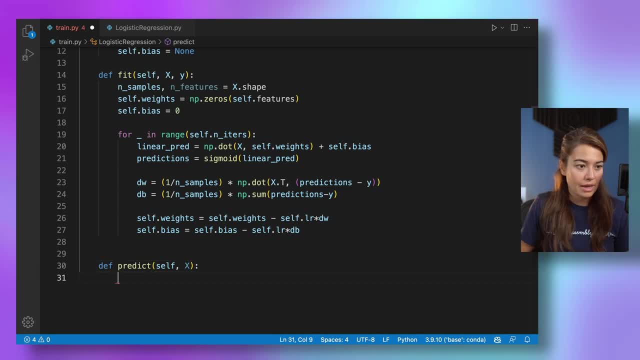 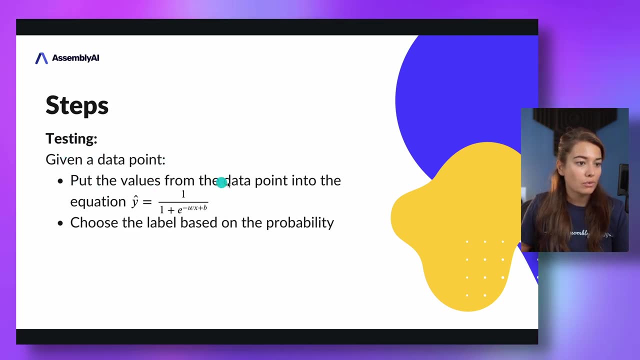 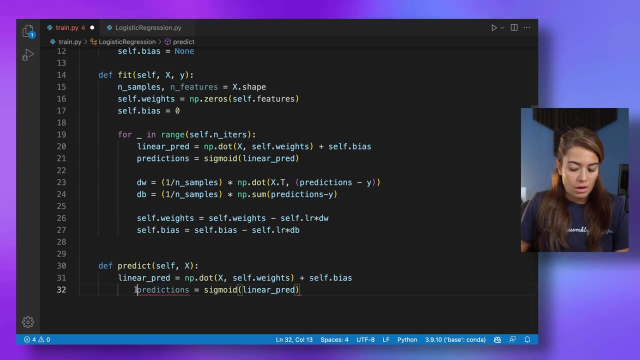 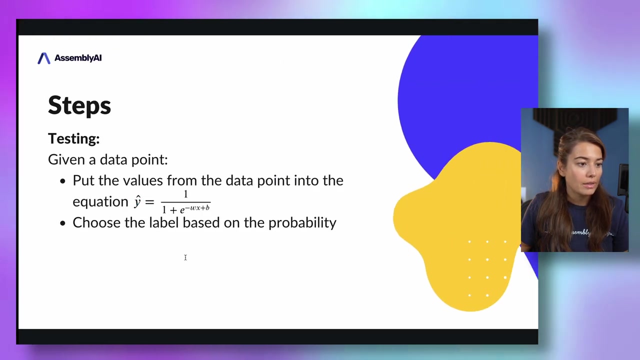 we need to pass it a set again. let's see how we did it here for the inference time given a data point puts the values from the data point into the equation, so we can just copy and paste this. actually I call this y pred for now. if we do the calculations here, all right, next thing: choose. 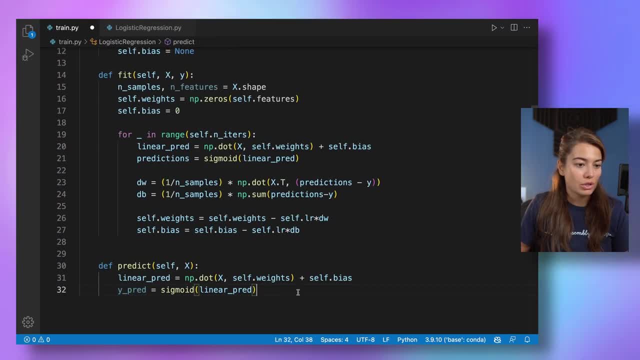 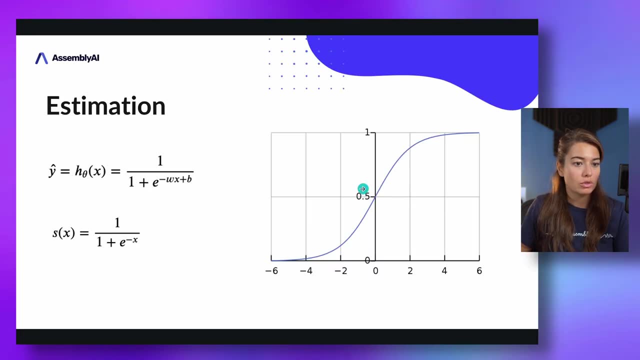 the label based on the probability. okay, so what we have in the predictions is the probability, of course, if we take a look at what the sigmoid- the results of the signal function, looks like, if we're going to have values changing from zero to one, basically. so what we're going to say is: 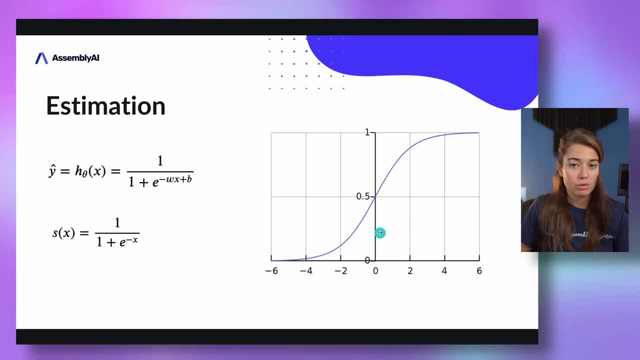 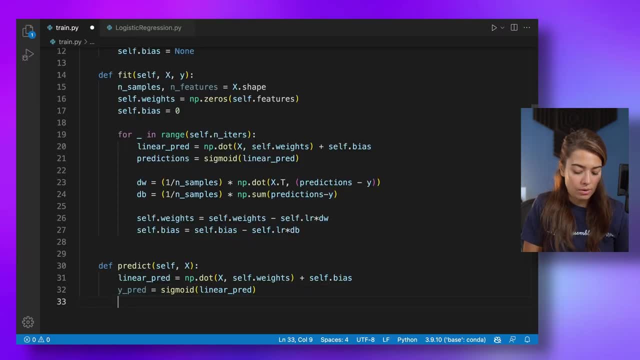 if it's between zero and 0.5, it's going to be zero. the label will be zero. if it's going to be between zero and five, 0.5 and one, it's going to be another label. so let's do that here for every. 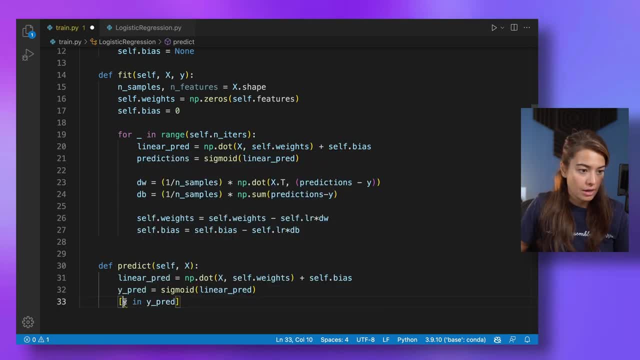 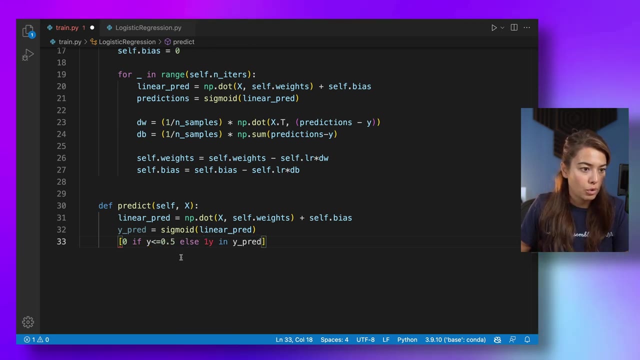 y in y predicted, the results should be 0.5 and 1 is going to be 1.5 and 1 is going to be 0.5 and 1 is going to be be 0 if y is smaller than 0.5, else it should be 1.. Maybe let's say smaller or. 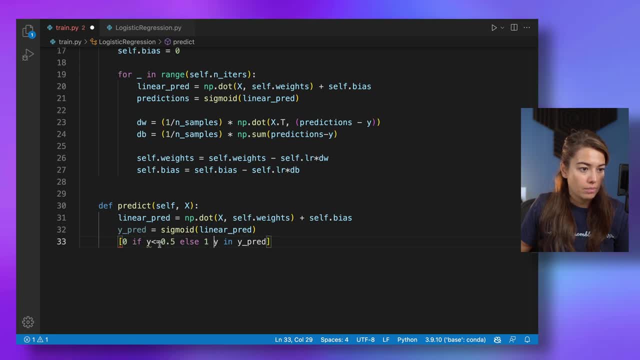 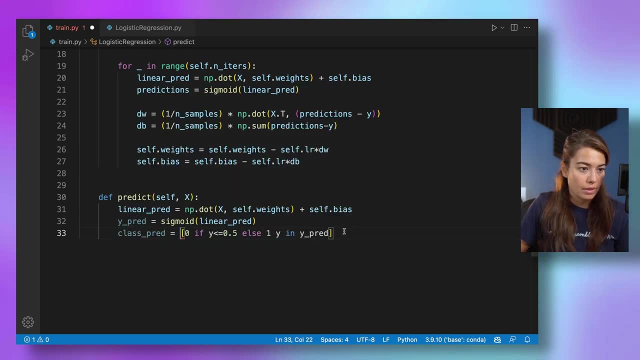 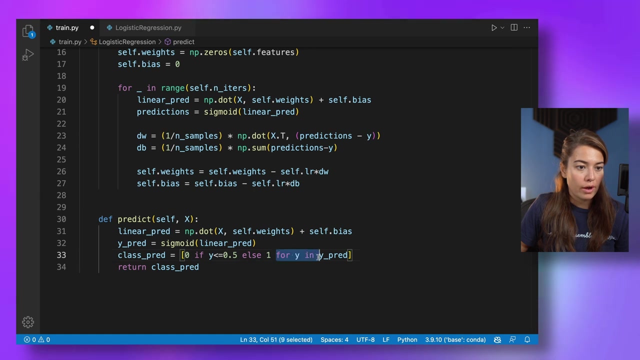 equal to 0.5.. Put it in the wrong place And this will be the class predictions, And then we can return this to say 4, of course. So for every y in y predictions, we assign them the value of 0 if the probability 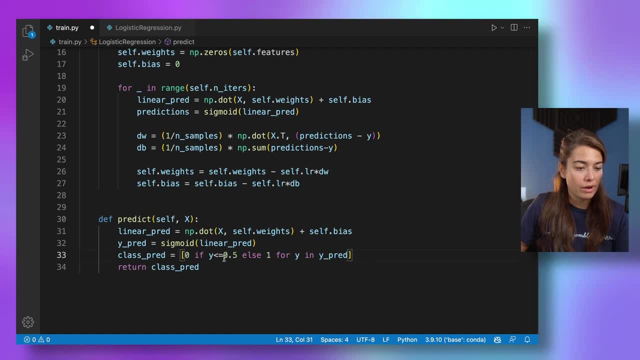 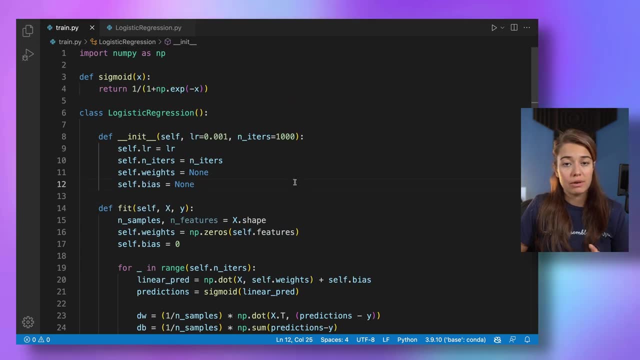 value is lower than 0.5 or equal to 0.5, otherwise it's going to be 1.. And then we return this Alright. so this is all with logistic regression. If you watch the linear regression video, you might realize that they're actually quite. 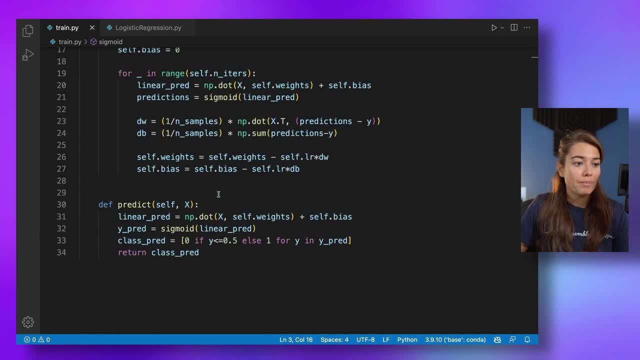 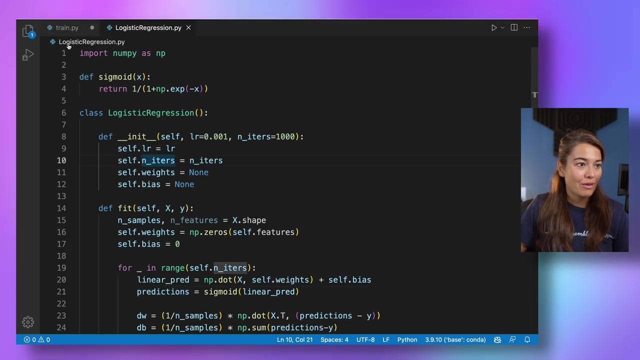 similar. The only difference is the addition of the sigmoid function and the calculation of the class labels after the probability is calculated. And oh, it looks like I wrote it down in the wrong file. I'll just copy, cut and paste it here in the logistic regression And in the train file. I'm going to see how. 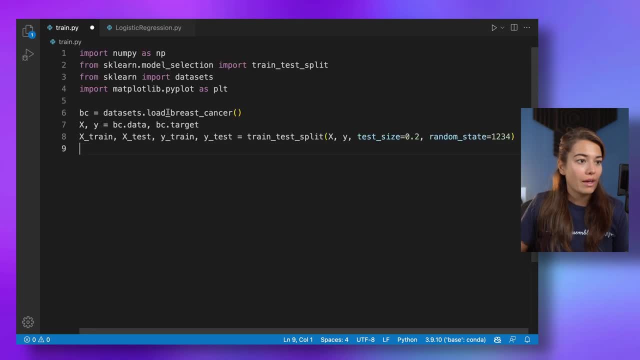 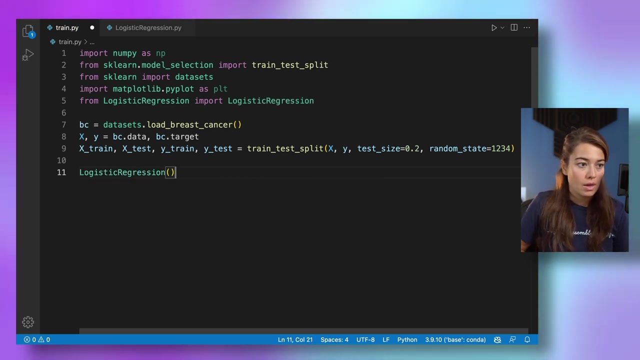 accurate. this logistic regression algorithm is For that. I am loading the breast cancer data set from scikit-learn datasets And I need to import logistic regression here. Alright, I'm going to create an instance of it And we can keep the original values. for now, This is going to be a classifier, And then I'm going to fit this classifier with the. 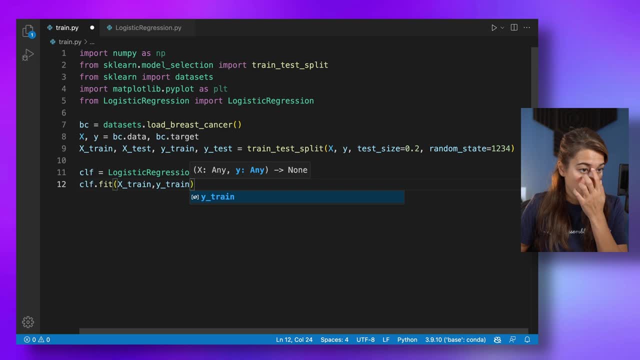 with the X train and Y train, and then we get the predictions: predict with X test values, and this will be Y pred. Alright, I want to report on its accuracy too, of course, so let's make a function that will calculate the accuracy for us. so it will be Y pred and Y test, and what I wanted to do is to tell me how many.